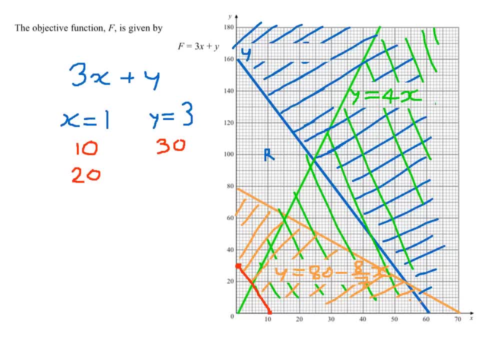 So, for example, I could double these, I could plot 20.. I could plot 20 and 60,, just to give me a bigger line. And again, y is 60,, x is 10, and you draw a nice objective line. 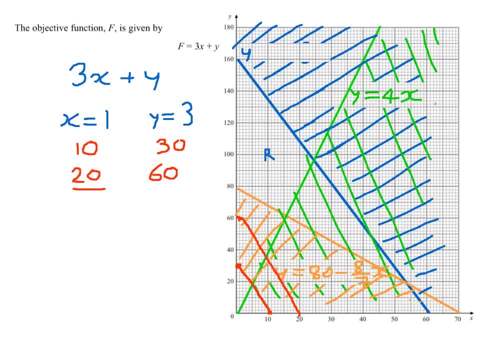 Now I have seen textbooks that tell you to keep multiplying these numbers and plot lots of objective lines across the graph. If you're doing an A-level paper, for example, they only expect to see one objective line to get the marks for the question. 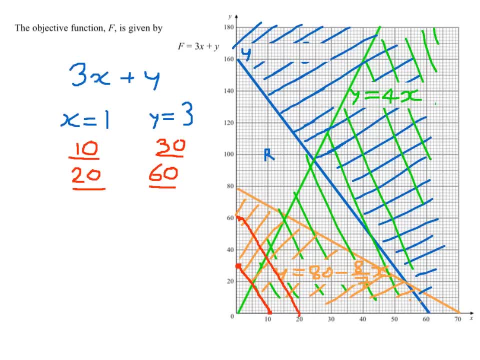 But they have to see that objective line on your drawing. What we're then going to do is take out our roughness. We're going to need a ruler, You're going to need a nice big ruler, And we're going to use this to find the optimum point on my graph. 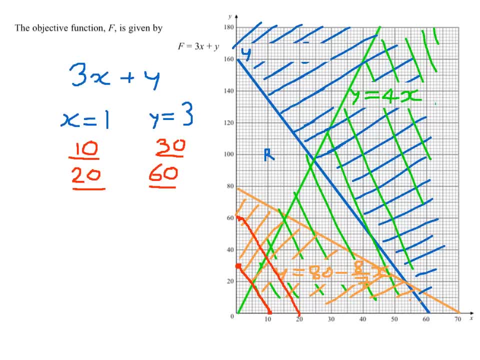 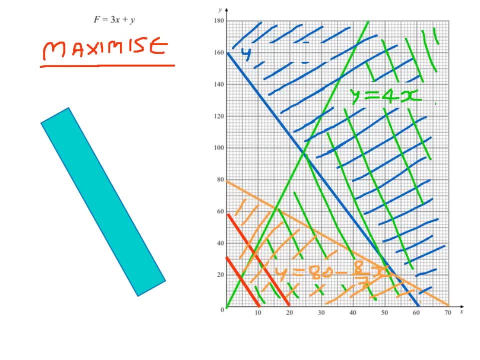 And that will depend on whether I'm finding the maximum or the minimum. So let's look at the situation where I want to maximise the function. I'm looking for the best values of x and y to give me the biggest value of f. 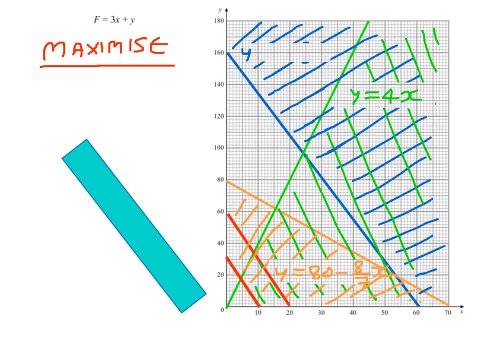 So I've taken my ruler here And what I'm going to do, I'm going to line up my ruler with my objective lines And you can see that if I've drawn those two, If I've drawn those two accurately, the ruler will line up perfectly with the two of them. 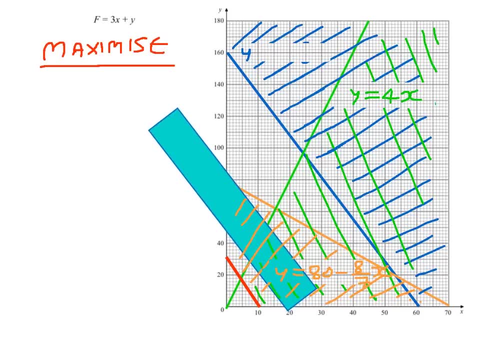 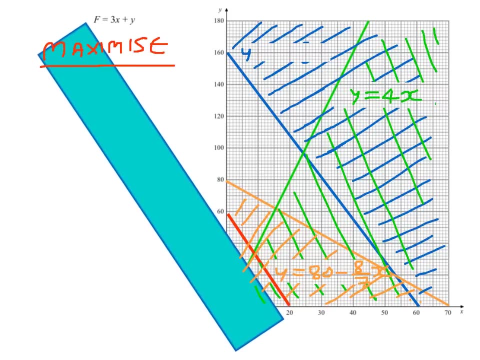 And what I'm going to do is I'm going to carry on moving my ruler across the page until I get to what will be the biggest point. Now you can see here, a 30cm ruler would be a lot better, Because then I'll be able to move it across the page. 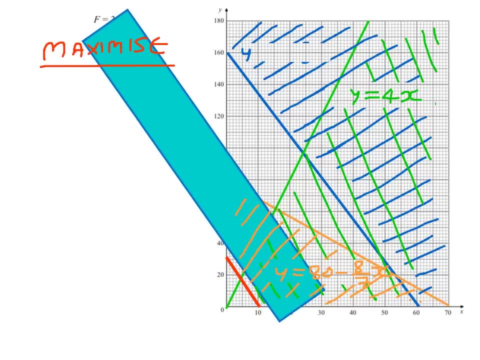 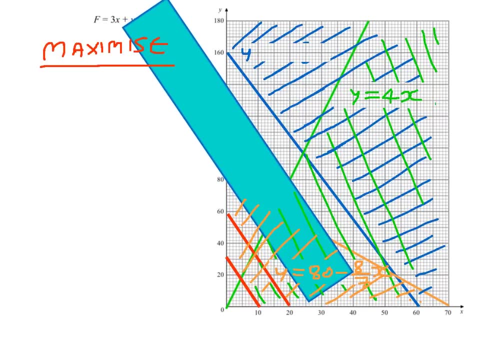 And if I'm maximising, I'm going to keep going until I get to the last point And making sure your ruler is lined up with your objective line at all times. So you see, it's still lined up there And I'm going to keep moving across. 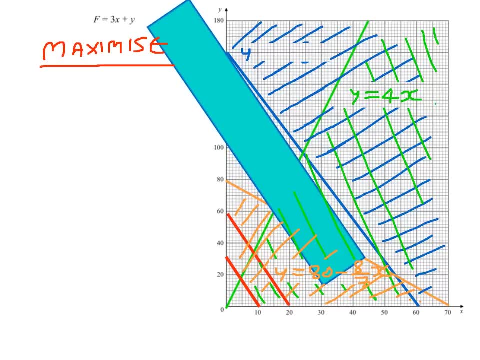 Okay, And I've got to be very accurate. You see, I've come and I keep moving. I can still see the region of my graph, Still see the region of my graph And there, If I just leave my ruler there for a second. 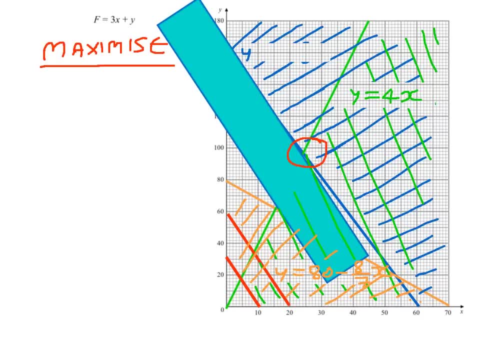 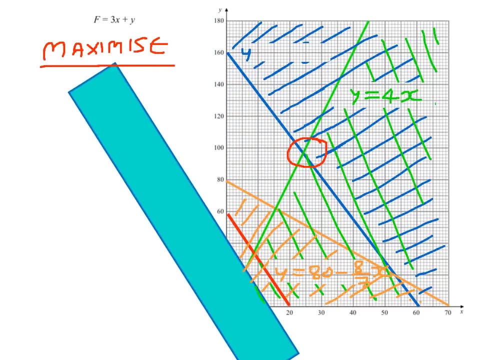 The last bit of the graph I can see is this corner here. Okay, that's the last bit of the graph that I can see. If I just pull my ruler away now, You can see that I moved it across And you can see my region. 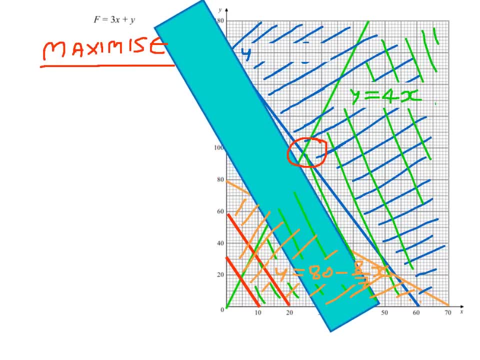 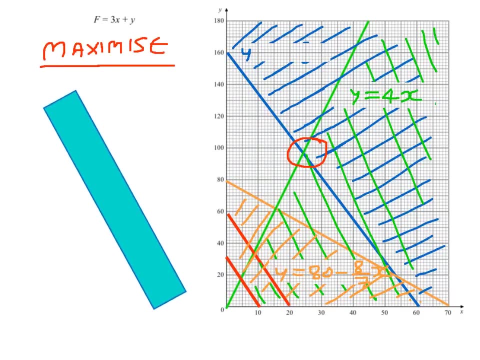 I'm in my region, In my region, In my region. Moving across, I can still see my region And there it's disappeared from view. Okay, So that was the very last corner. So that's going to be the answer to my maximum function. 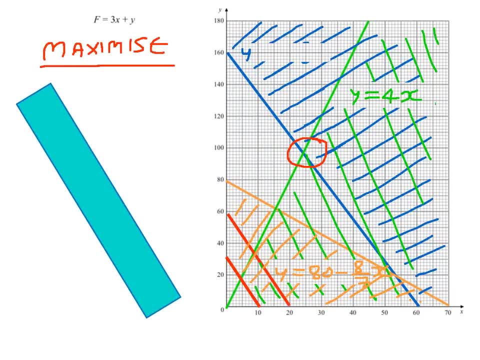 I need to find the values of x and y from that corner, And therefore I can maximise my function. So let me do that now. Now, the important thing to realise is that the corner I've selected lies on the lines. Get a thinner pen. 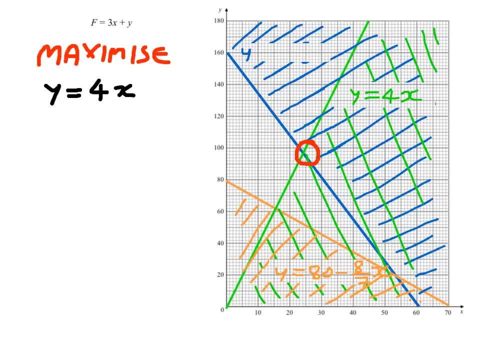 y equals 4x, And it also lies on the line: y equals 160 minus 8 thirds of x. Okay, These are solid lines, So it's absolutely fine. It lies on those lines. It can equal that. Now, all I do is solve this simultaneously. 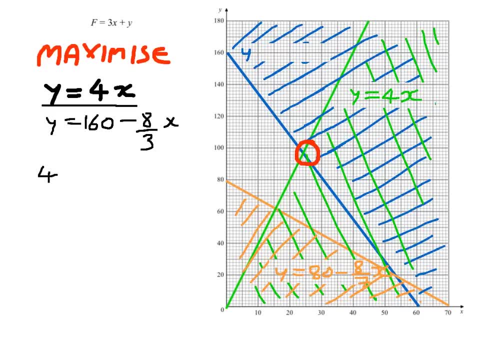 So I'm going to sub that first equation: y equals 4x in. So instead of y I write 4x equals 160 minus 8 thirds of x, And if you've got a calculator you can probably do this a lot quicker. 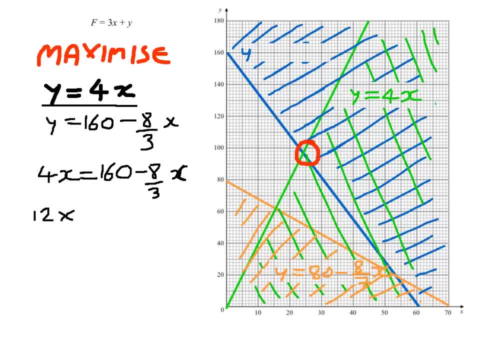 I'm going to do it by hand, So I'm going to times everything by 3.. 12x equals 480 minus 8x. Just to make my life easier, Bring the 8x across. So 20x equals 480. 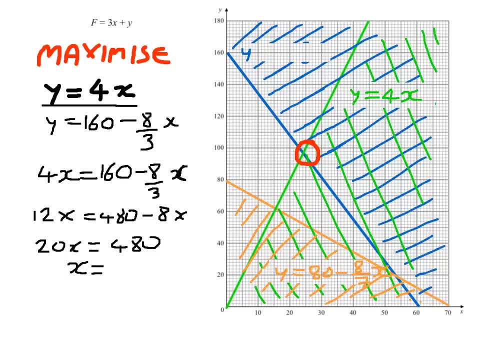 And therefore I can get my answer: x equals 480 divided by 20.. And you should get: x is 24.. Now you're absolutely right. Some people are saying: I have read that off the graph And you can see there. 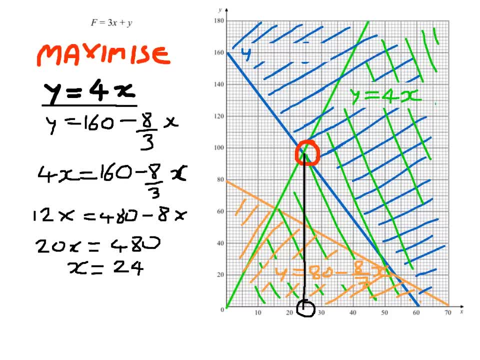 x does indeed equal 24.. But you need to be very careful. You'll often be drawing these graphs by hand in an examination situation And you can't guarantee you're that accurate between could this have been 23,, 23 and a half? 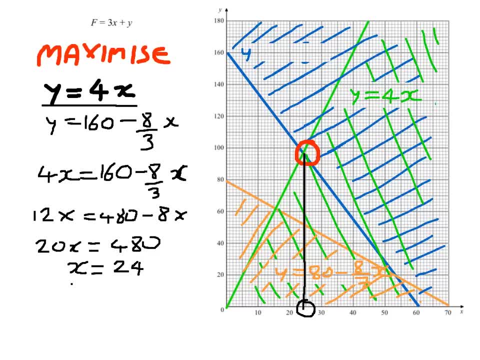 So you need to be very careful. y just equals 4, lots of x, We've seen that. So y is going to equal 24 times 4.. So that's 48 doubled is 96.. And lo and behold, if I look at my graph. 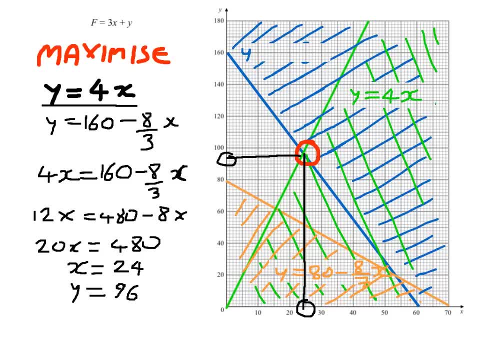 it should be around 96.. The question wasn't find x and y, It was maximise your function. Well, now you're just subbing your values, So f is going to equal 3 times whatever x is, Which is 24.. 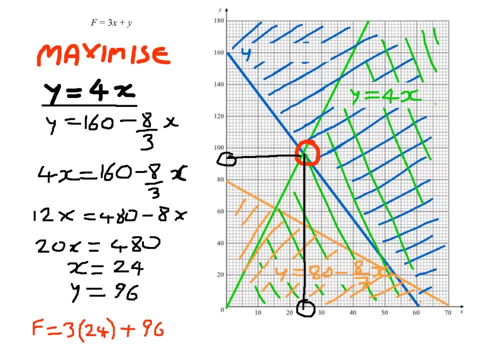 And then plus 96.. You do that on a calculator And you get an answer. I don't have a calculator on me. I should probably pause and go and get one, But you can see this is going to be. you can see this is going to be 168. 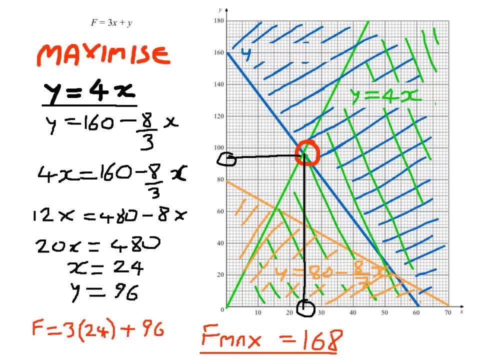 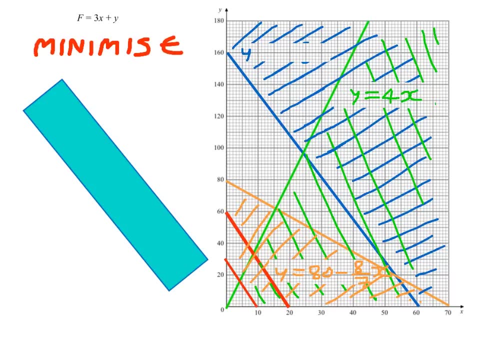 Tell me if I'm wrong. And that's f of x maximised. So let's see what happens if we minimise. It's exactly the same process, But we're going to minimise the function this time, Which sometimes also comes up, So going back, getting our ruler again. 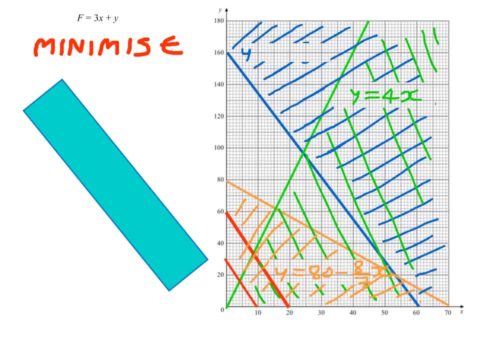 Ideally a 30 centimetre one, One that can fit across the page. It's these little things that make a difference in an exam. So get yourself down to power land 99p store. You'll be able to get a 30 centimetre ruler. 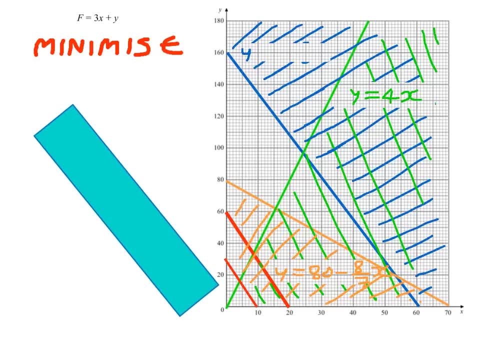 For presumably 99p or a pound, Get your mum to go and get you one And then take your ruler And what's the first thing we do? We're going to line it up with our objective line. So I drew two lines. 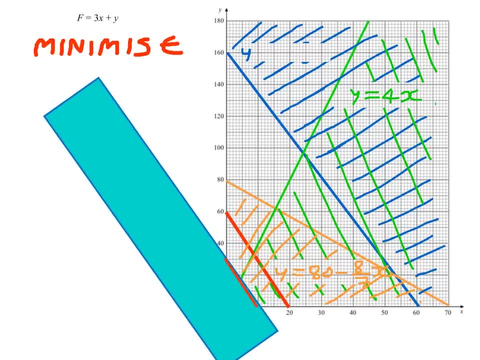 I drew that one, But I also drew one there And of course if you draw them correctly they'll line up. So we're lining the ruler up nicely like that. Now I'm looking for the minimum value. So in my region, R. 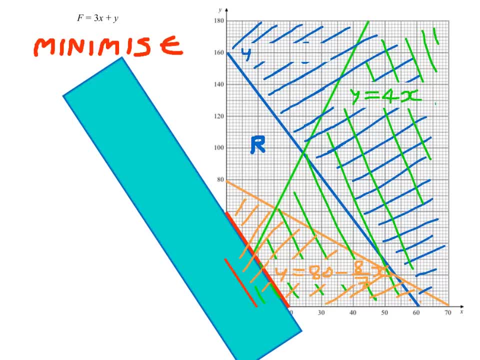 I'm looking for the very first value I come to. So if I take my ruler- Okay, we're just jumping about all over the place- I'm going to slowly slide it across the page, Staying lined up with my objective lines. 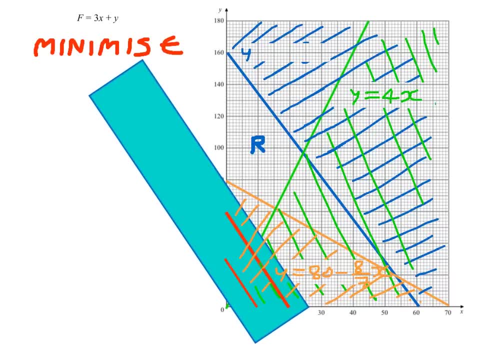 And there I've got the very first value I've come to. You should all be able to see that there, This vertex, here, this corner, is the very first value that I have come to. So that's where my values of x and y are going to come from. 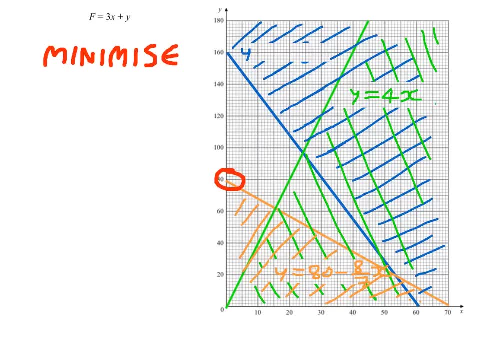 for the minimum value of f. So now we've got our first value. So now we've found the vertex where the minimum value lies. It really only lies on one line, And that's the orange line in this case, which is: y equals 80 minus 8 sevenths of x. 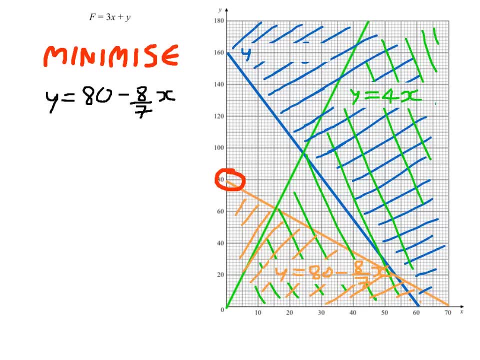 Of course, the other line it lies on is the y axis, which, of course, is sometimes known as the line x equals 0. Obviously, at this point here, x equals 0. So all I need to do is sub 0 in. This is pretty trivial.